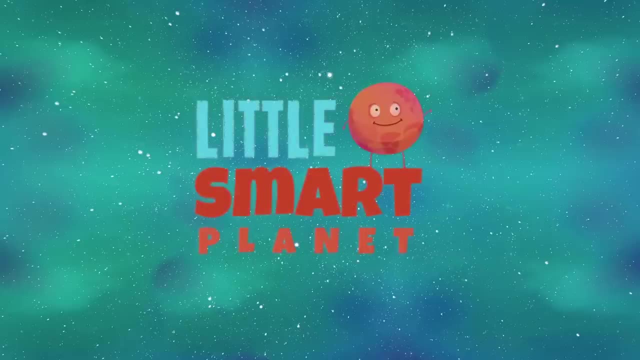 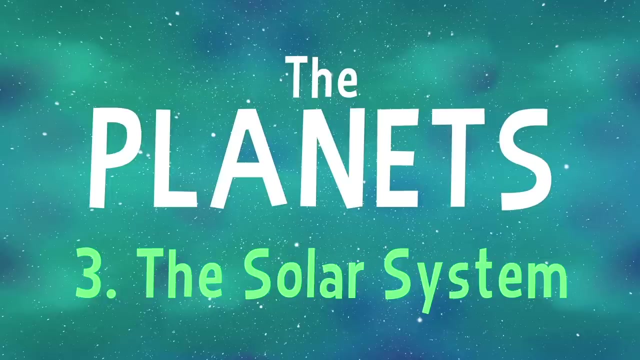 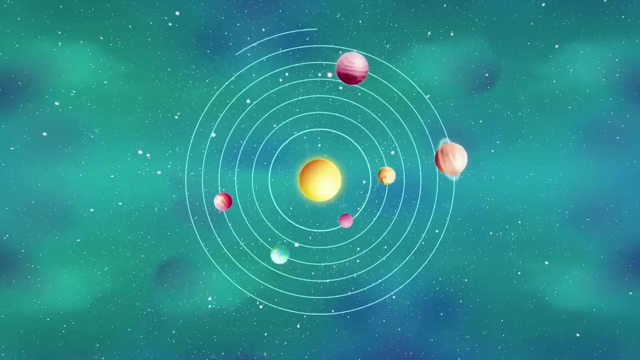 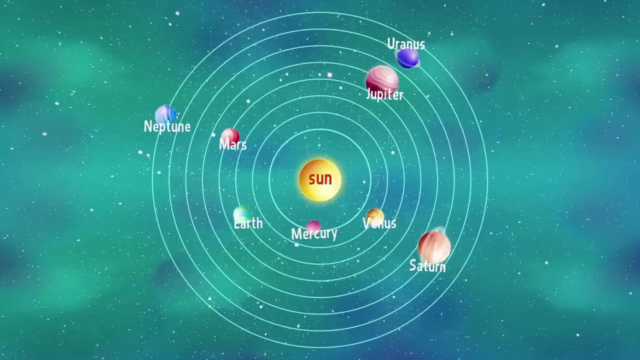 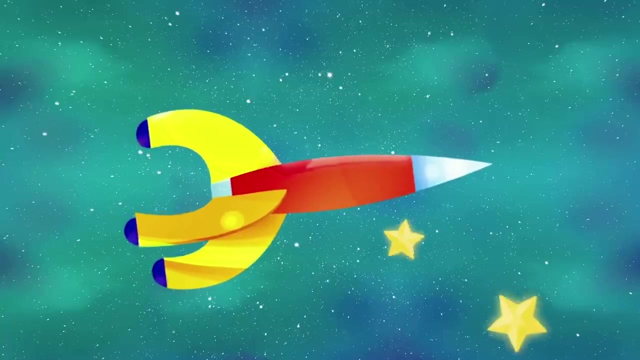 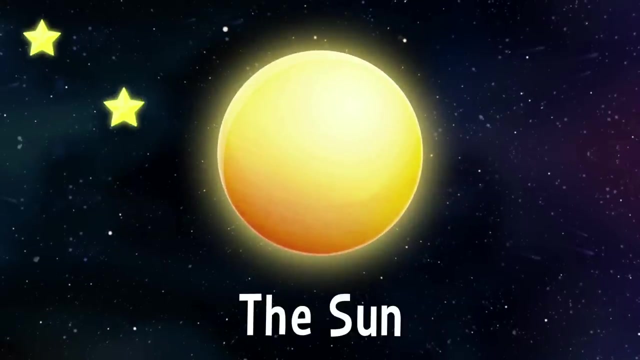 This is our solar system and we are taking a tour around it. Right at the center is the sun. It's much bigger than the planets that spin around it. Now we are going to jump into our spaceship and see all the planets in the solar system. Come with me. The sun is a star. 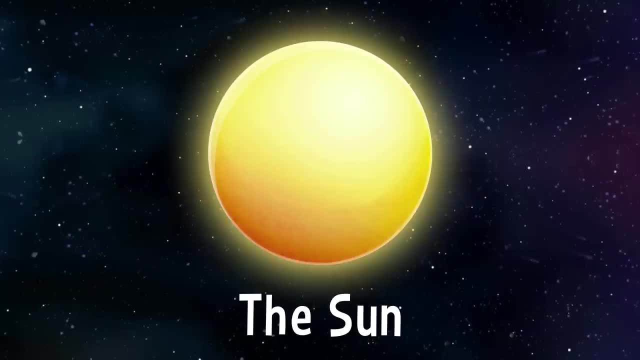 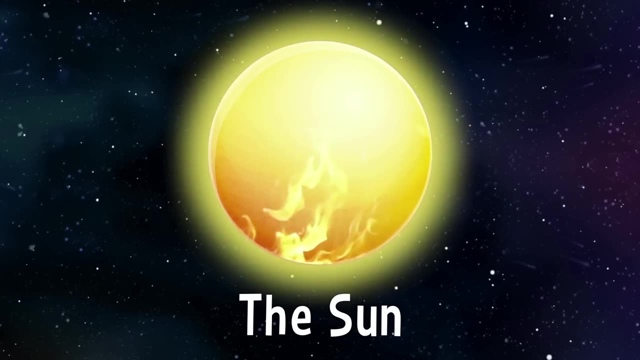 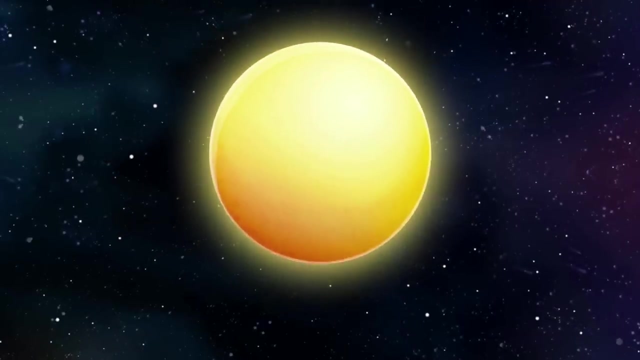 and it's really big. It's 100 times bigger than the Earth. It's a ball of fire. That's why it shines so bright and gives us heat. Don't get too close to it or you'll get burnt. Goodbye sun. 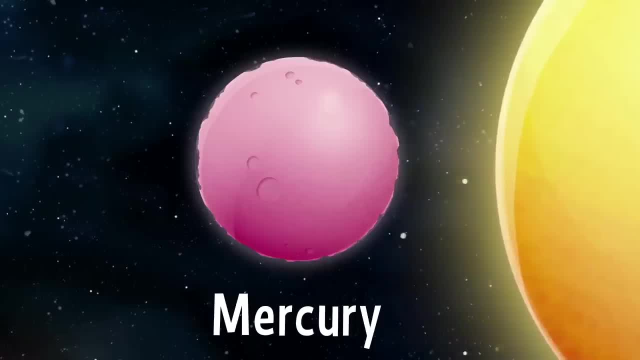 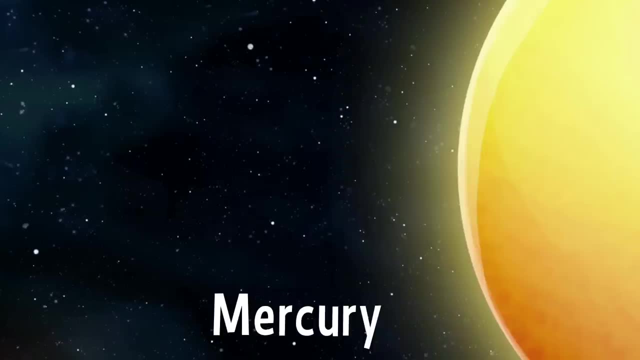 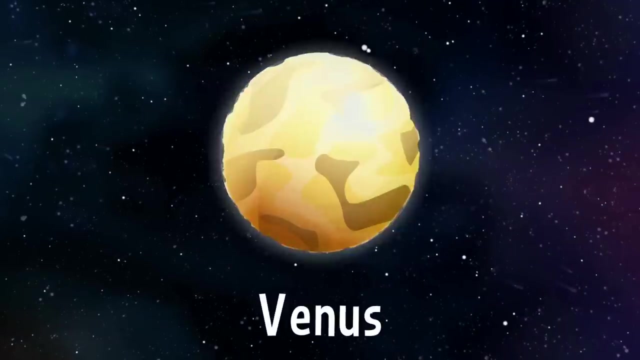 Mercury is the closest planet to the sun and it's the smallest planet in the solar system, But it is also the fastest to spin around the sun. See you soon, Mercury. Venus is the second planet after the sun, but it's also the warmest. It is yellow and 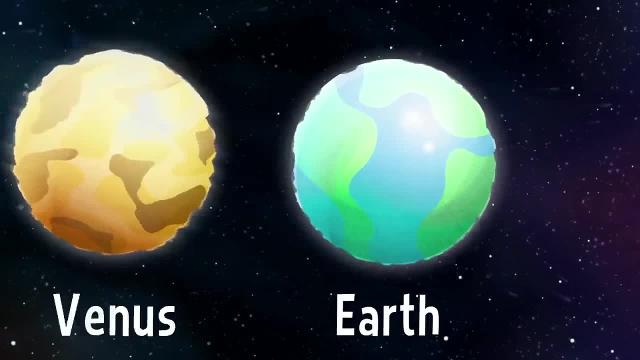 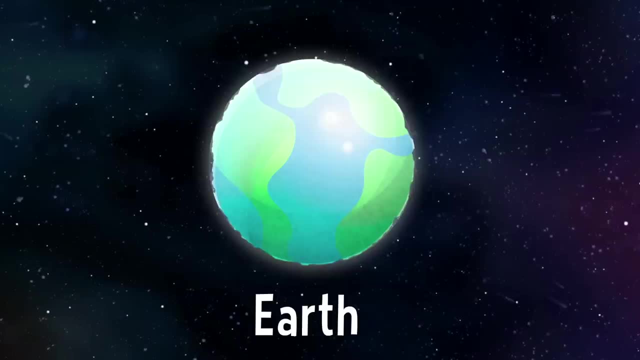 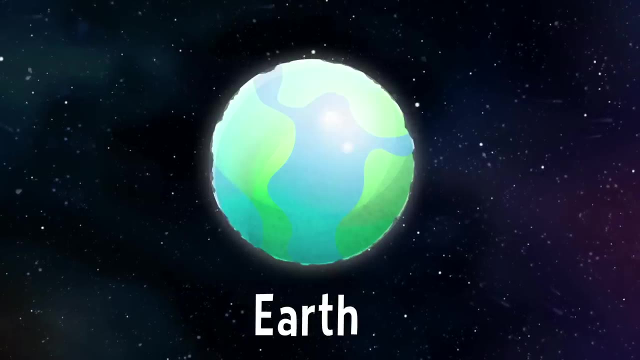 it's the same size as the Earth. Earth is our planet. It's where we live. It looks beautiful from far away, All blue and white and green, from the sea, the clouds and the land. It's the only planet with life in our solar system. That's why it's so special. 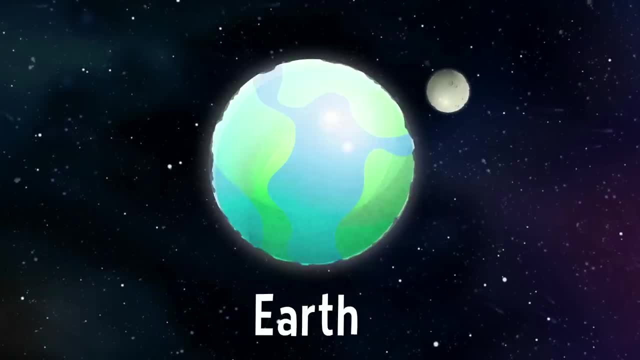 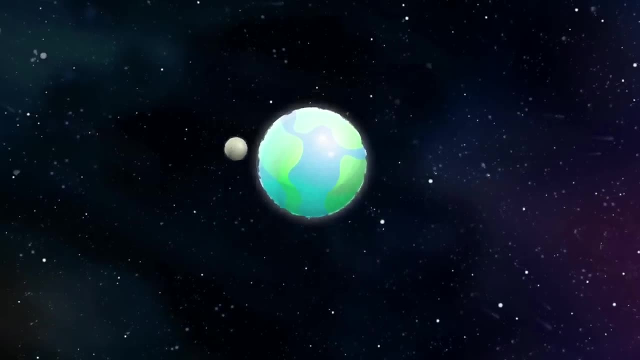 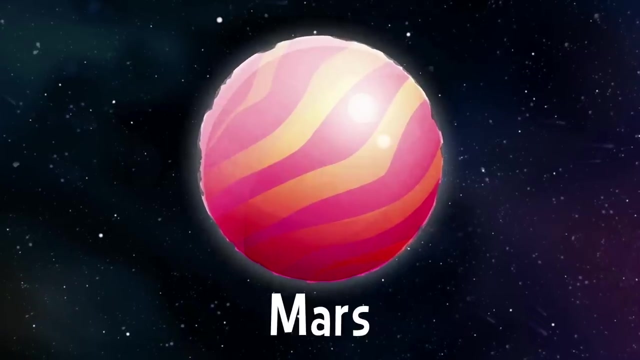 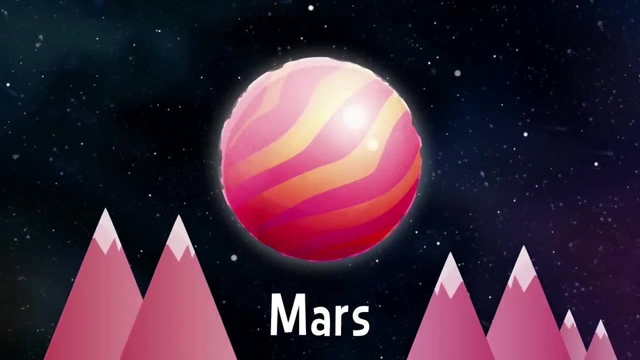 Oh, look, There's our moon. It spins around the Earth, Isn't it beautiful? Bye, bye Earth. Mars is the fourth planet in the solar system. It is sometimes called the red planet. Mars is made of rock, And there you can find the tallest mountains in the solar system. 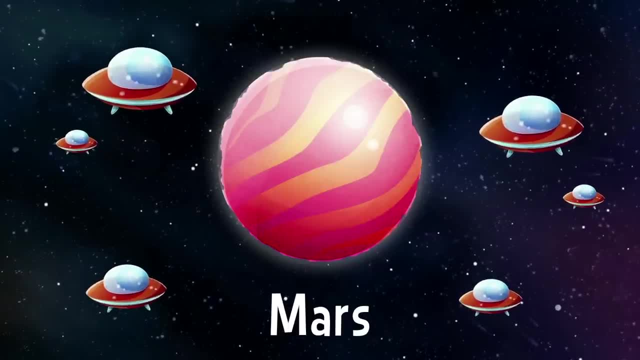 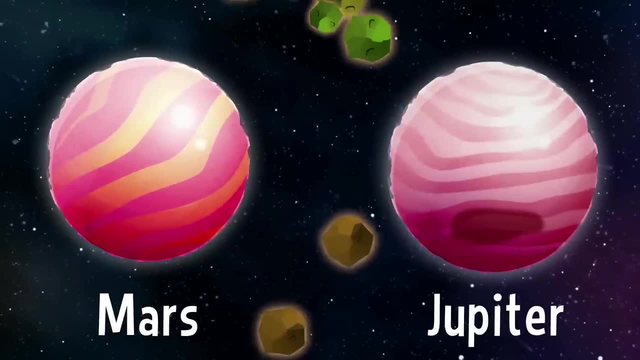 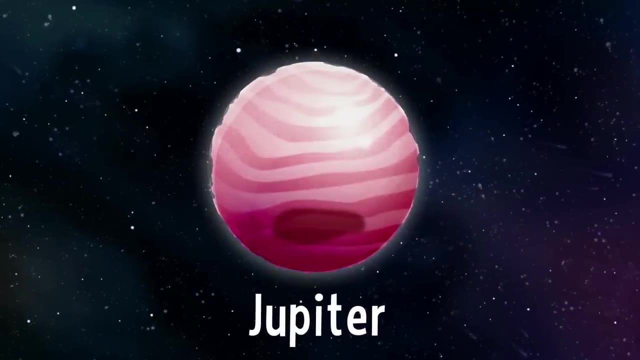 Also, Martians are from here. No, I'm kidding, There are no Martians. Careful, Between Mars and Jupiter, there is a giant asteroid belt. Jupiter is the fifth planet of the solar system. It's the biggest of all and it's made of.